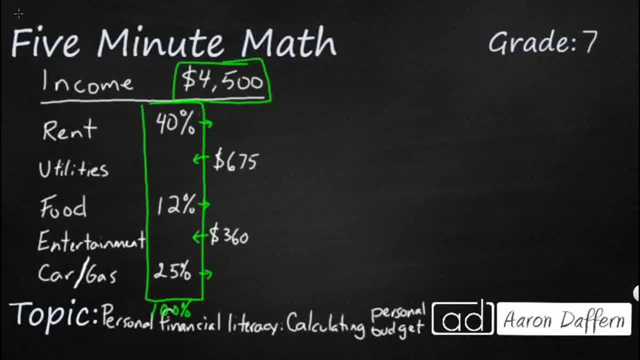 So let's just start with our percents. We'll start with that real quick. So rent is 40% of our total income, 4,500.. So what does that mean when we're taking 40% of something? Well, 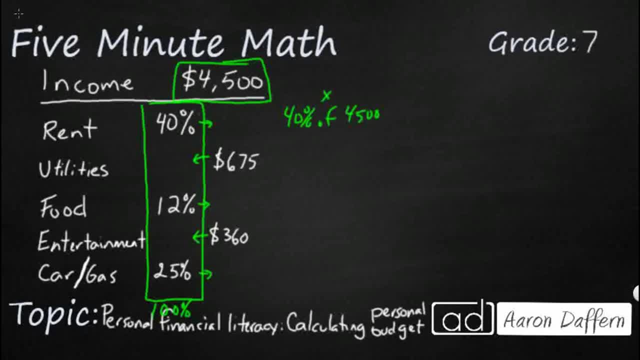 of means. we're going to multiply that 40% times 4,500, but we need to change that percent into a decimal. So let's figure out where our decimal point is going to be. It's after the ones place. If it's not already there, we're going to move it over twice left. So 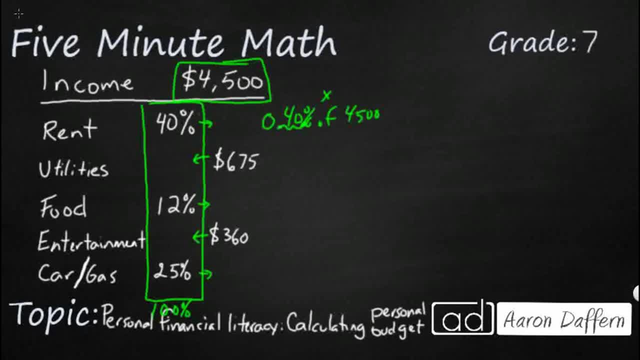 really it's 0.40, or we can just think of it as 0.4, because four tenths and 40 hundredths are the same thing. So let's just multiply. When we get the decimal, we can go and multiply. 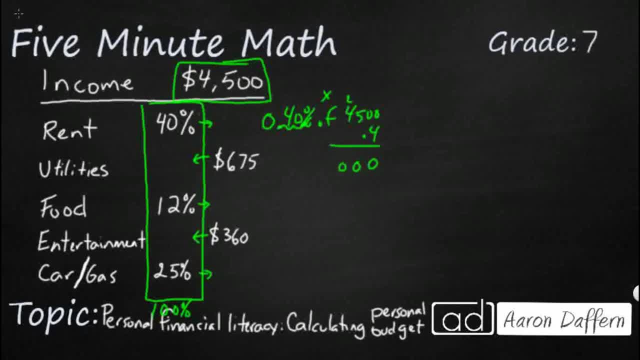 that zero, zero, that's 20.. And that is going to be 16,, that's 18.. One digit behind the decimal in our factor, So one digit behind the decimal, Okay, In our product. So it's $1,800.. So a lot of rent, That's 40%, not quite half getting. 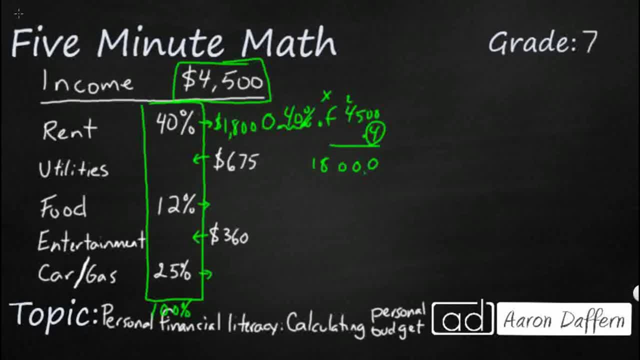 kind of up there. So you've got our $1,800 right there, So we can do that same thing for food. So we need 12% of our 4,500.. Make sure we're always doing it of the total There's. 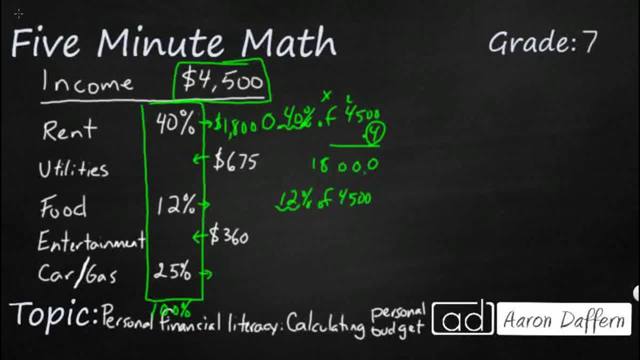 no decimal there, So we put it after the ones place. move it over twice. once twice, 0.12 is the same as 12%. So let's just multiply that Zero, zero, I've got 10.. Eight, that's nine. Next. 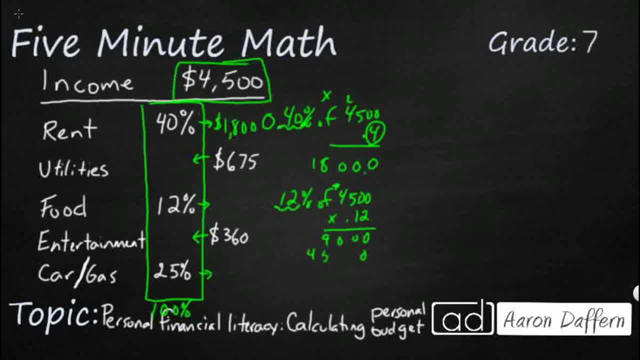 row And then let's just copy down my 4,500.. Add that up here. That's going to be 14.. And that's All right, 54.. Let's make sure we've got two digits behind the decimal in the factor Two. 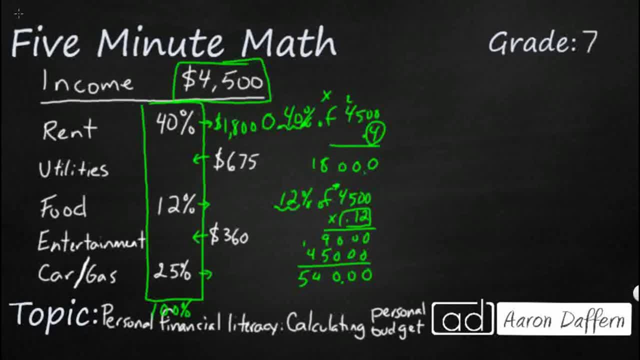 digits behind the decimal in our product. So we've got 549.. Not nearly as much as that. 40%, if that makes sense. So I'm guessing. Look at this: Car gas is 25%. That's a little bit more than double, So I'm guessing that's going to be.